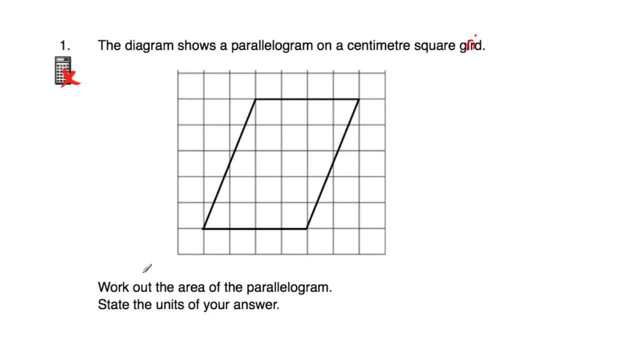 squares measures one centimeter by one centimeter, and we're asked to work out the area of the parallelogram and to state the units of our answer. So there's a few different ways we can do this. One way is to count the number of whole squares, so one, two, three and so on, and then put part squares. 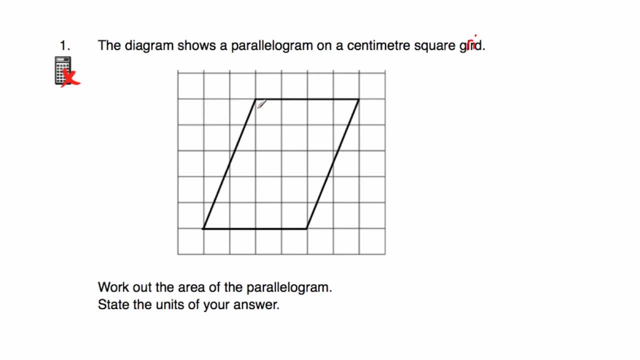 together to make whole squares and so on. So that's one way you could do it. Another way you could do it is to chop off this part, this triangle, and put it on this part, and then you've got a rectangle and then you can work out the area. Alternatively, you could use the formula, So the area for 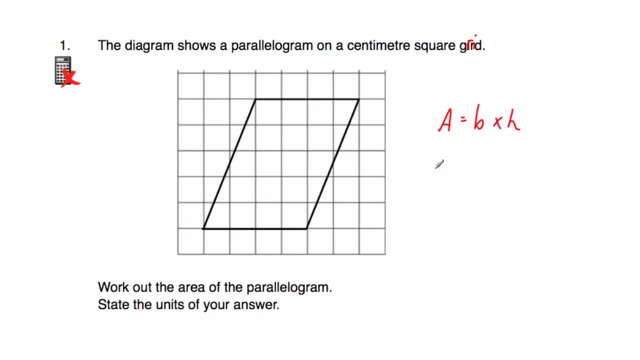 parallelogram, the area is equal to the base multiplied by the square. So the area for parallelogram, the area is equal to the base multiplied by the height or the perpendicular height of the parallelogram. So if we look at this parallelogram, 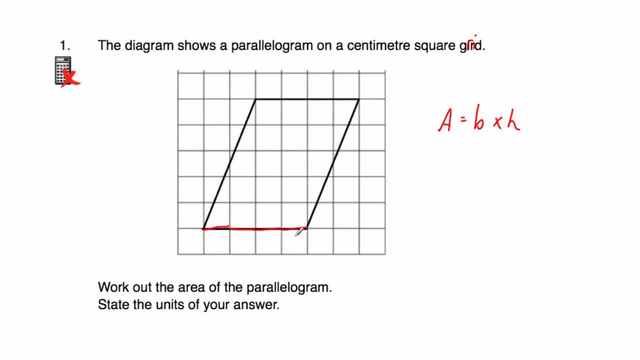 the base is one, two, three, four centimeters long, so four centimeters The height of the parallelogram. well, it's got a height off. if we go up from the base to the top, it would have a height off if we go upwards- one, two, three, four, five centimeters. it's got a height of five centimeters. So if we just do, 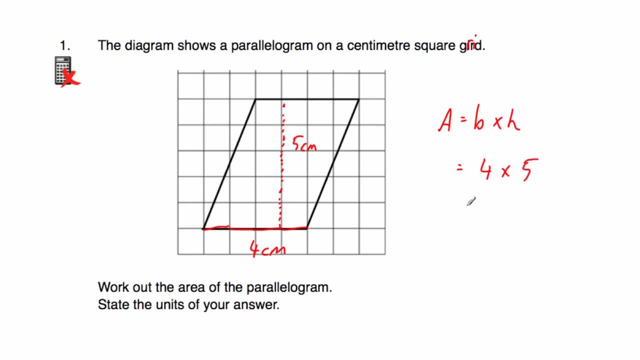 base, which is four, multiplied by the height, which is five, that will give us the area, and four times five is 20 centimeters squared, and that's the area of the parallelogram. Alternatively, you could have chopped this part off. so if I just get rid of this, Alternatively you could have just chopped- 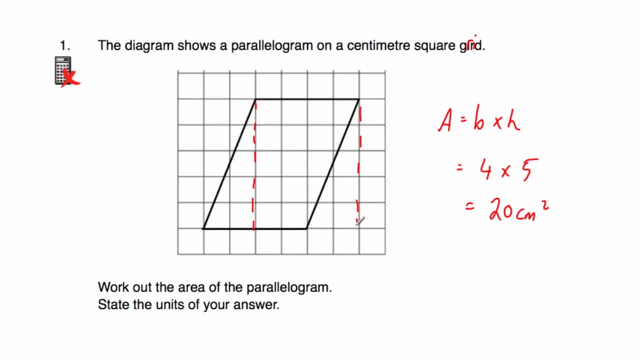 this part off here and put it on the end here, and then you would have had this rectangle and it's four by five. so four times five is twenty. But I like using the formula for the area of parallelogram because I think it's quite straightforward. base times the height. Okay, let's have a look at our 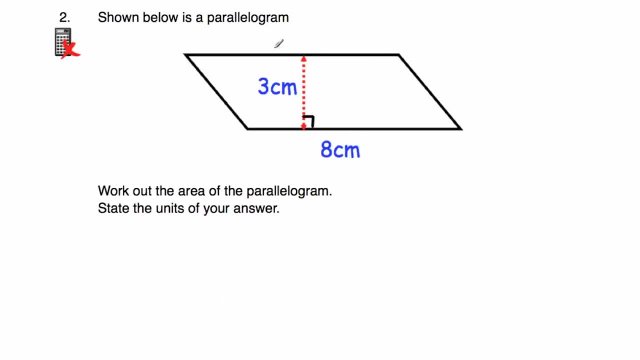 next question. So question number two says: shown below is a parallelogram. So we've got this parallelogram. it's got a length of five centimeters. So we're going to take the length of the parallelogram and we're going to. 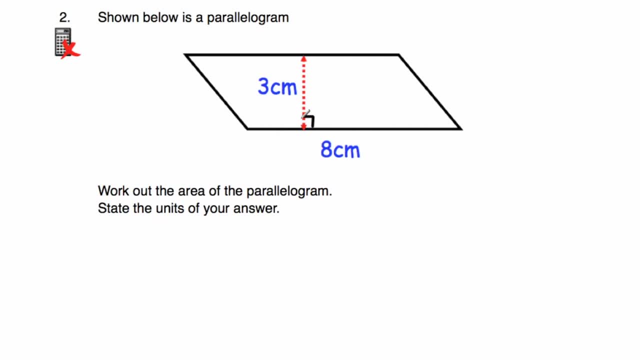 take the length of eight centimeters. So the length of the base is eight centimeters and it's going to height the distance between the base and the top of it of three centimeters. We've been asked to work at the area of the parallelogram, so we're going to do the base. so area equals base times. 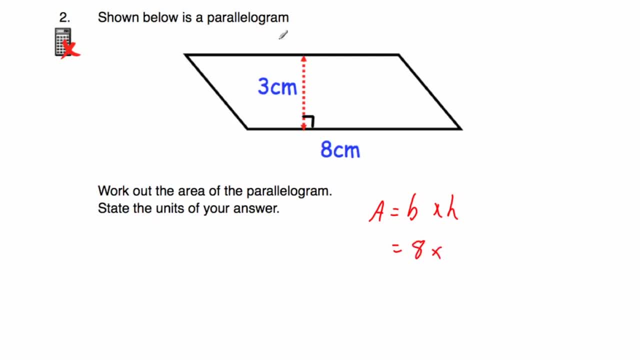 height. The base is eight centimeters. so eight multiplied by the height, which is three, and eight times three, is 24.. And we've got to make sure we put our units on and because we're dealing with area of the shape and we're dealing with centimeters, it's going to be centimeters. 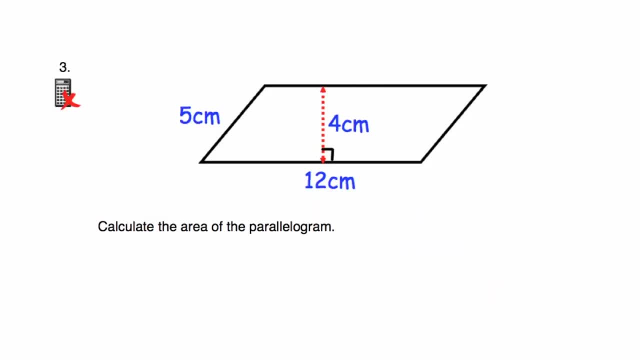 squared. Okay, our next question, question number three. So, question number three: we've been given a parallelogram and this parallelogram, we have got the base here of 12 centimeters, we've got the height of four centimeters and we've got the length of the diagonal here, the. 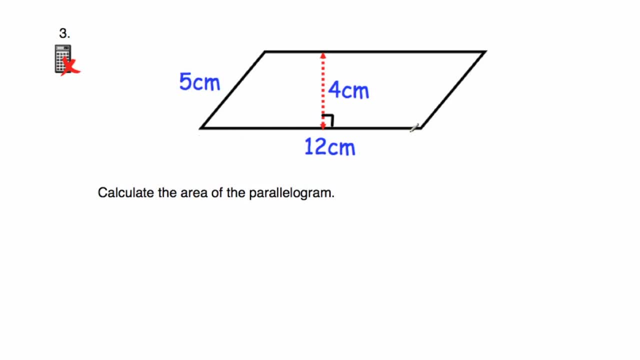 length of the side as five centimeters. Now we've been asked to calculate the area of the parallelogram, so we need the base and the height. so we're just going to do the base times the height. we don't need to worry about this five centimeters. This five centimeters would be useful if we're finding 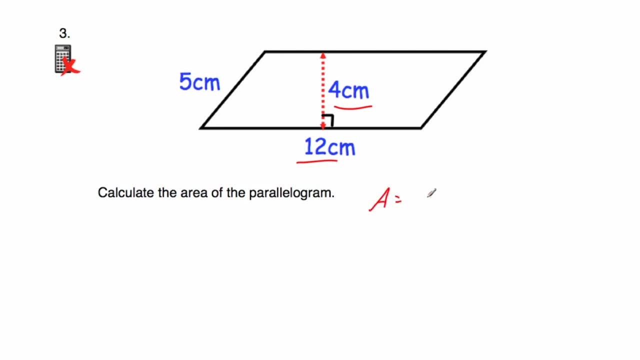 the perimeter of the parallelogram. but for the area of the parallelogram I'm going to do the base times the height, the perpendicular height, the distance between the base and the top of it. So the base is 12 multiplied by the height, which is four, and 12 times four is equal to 48 and make 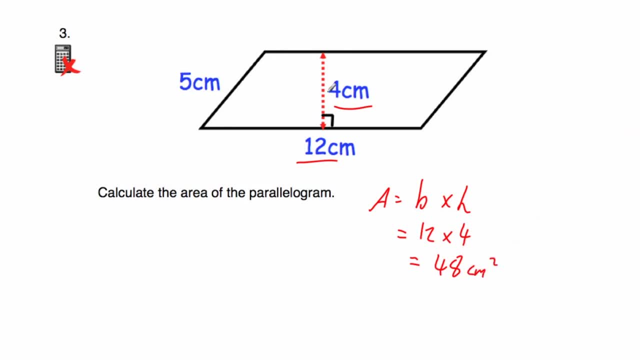 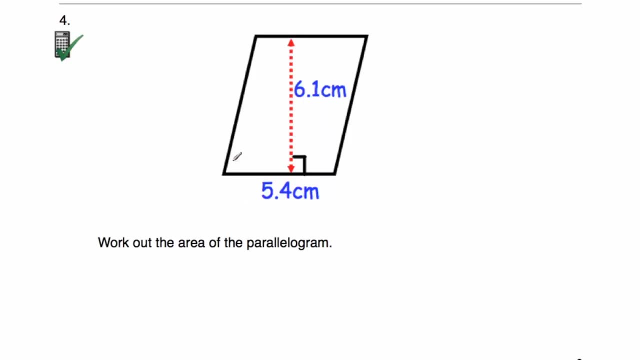 sure, we put our units on centimeter squared, and that's it. so the area of this parallelogram will be 48 centimeters squared. we can just ignore this length. Okay, our next question, question number four. a question number four is a calculator question and we've been asked to find the area of this. 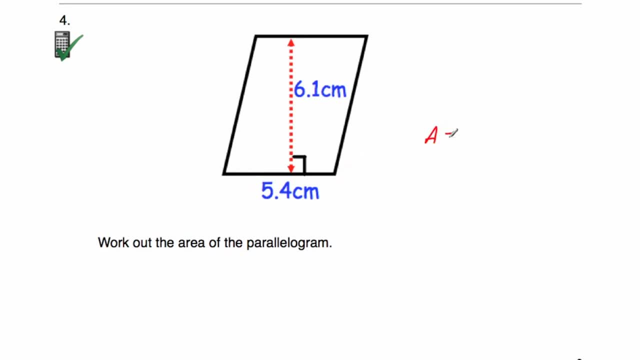 parallelogram. We've got its base, we've got its height, so we just need to. the area is equal to the base times the height. So we've got the area of the parallelogram and we've got its height, so we just need to. the area is equal to the base times the height. 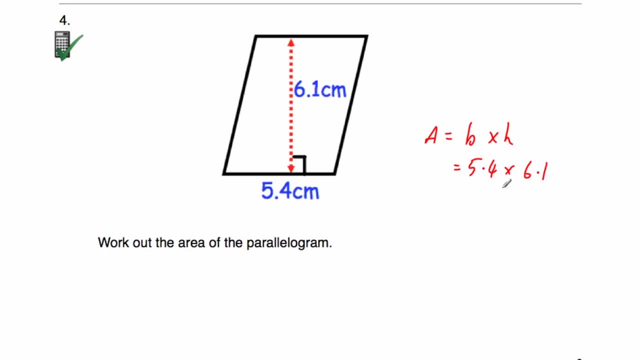 The base is equal to 5.4, the height is equal to 6.1 and if we multiply these on our calculator, 5.4 multiplied by 6.1, that gives us an area of 32.94 centimeters squared. and that's it, and just make. 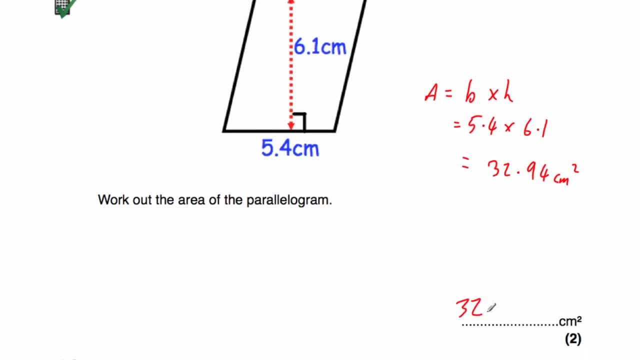 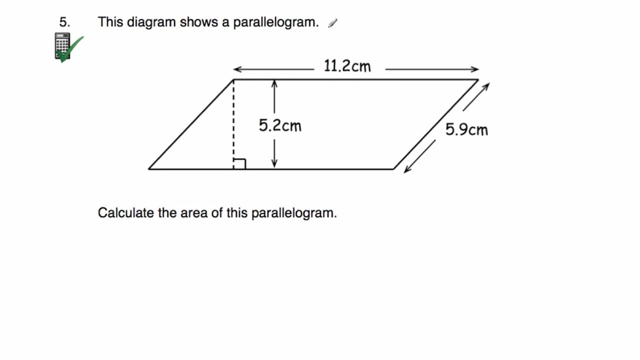 sure you put your units on if you need to. actually they're in the answer box here, so we just write 32.94 and that's it, Okay. our next question. okay, let's have a look at question number five. so question number five says this diagram shows a parallelogram. so here we've got a parallelogram. 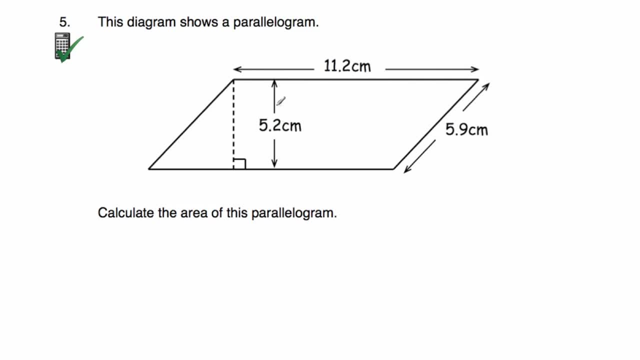 the parallelogram has got a length of 11.3 centimeters, height of 5.2 centimeters and the length of the side is 5.9 centimeters. now we're not going to need to use this, because we just need to do the base times the height. the base would be: 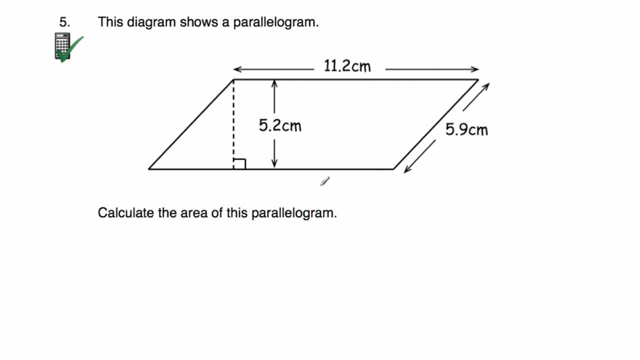 11.2, the same as the top times the height, which is 5.2. so we're going to do: area equals base times height. the base is 11.2, the height is 5.2 and if we multiply those together using our calculator, 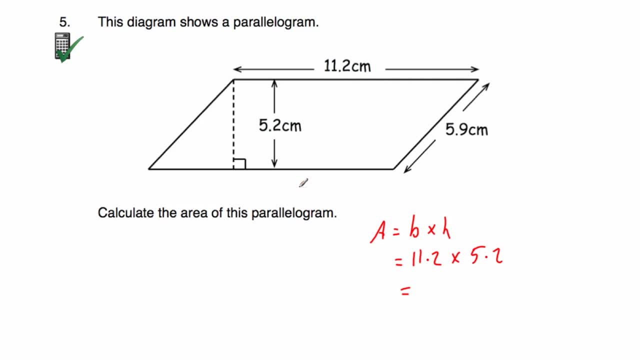 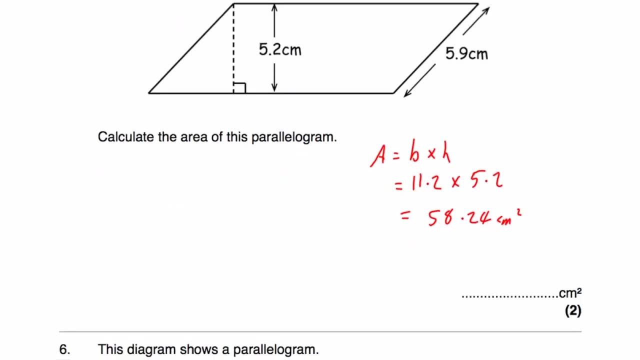 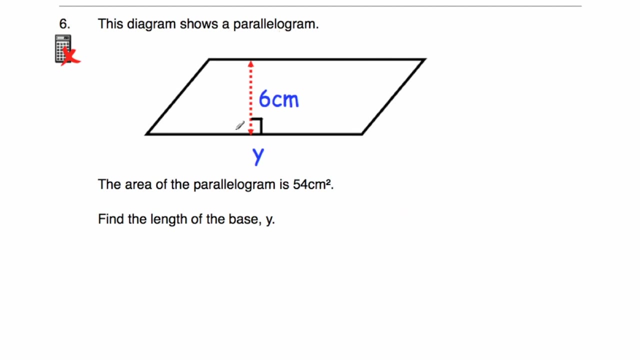 that will give us our answer. so 11.2 multiplied by 5.2 equals 58.24 centimeters squared. so that's the error of the parallelogram: 58.24. okay, question number six. question number six says this diagram shows a parallelogram. so we've got this parallelogram. 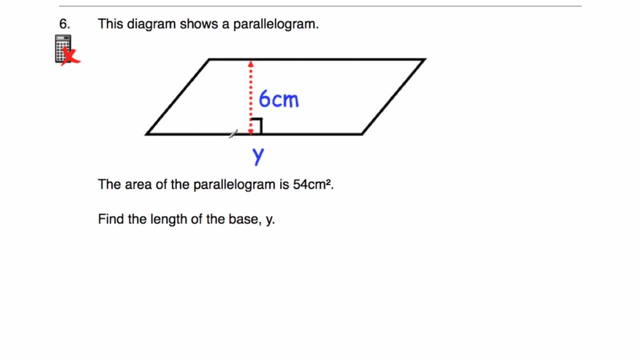 the length of the base is y and the height of the parallelogram is six centimeters and we're told the error of the parallelogram is 54 centimeters squared. find the length of the base y. so to find the area, we multiply the base by the height. so whenever we do this number y times 6, we get 54.. 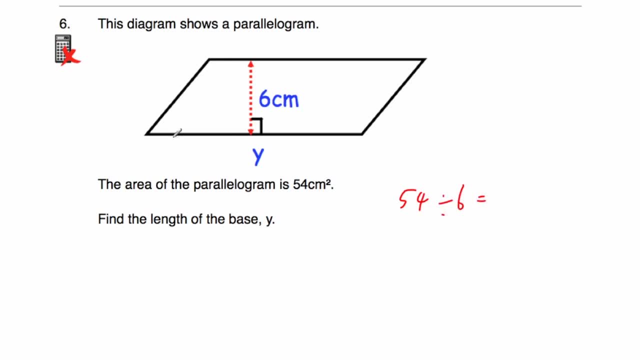 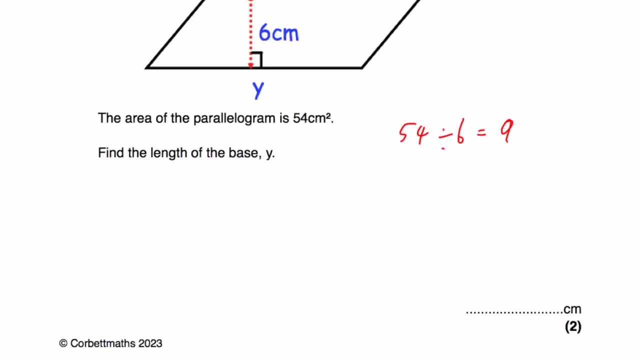 so if we do 54 divided by 6, that would tell us the length of the base. so 54 divided by 6 is 9.. so that means that the base would be y would be 9 centimeters. so the length of the base is 9 centimeters. so if you're given, 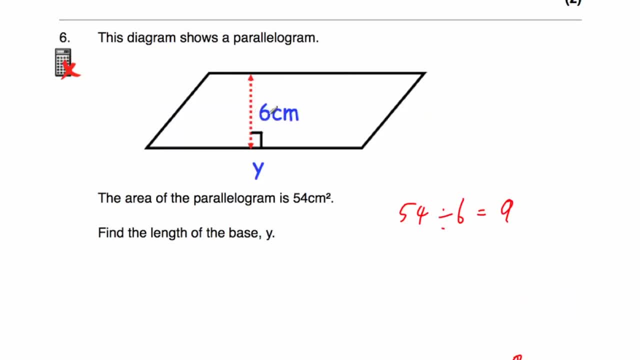 the area for the parallelogram and you know the height. if you divide the area by the height, you will find the length of the base. and likewise, if you were given the area and you knew the base, if you divide the area by the base you'll find the height of the parallelogram. okay, question number. 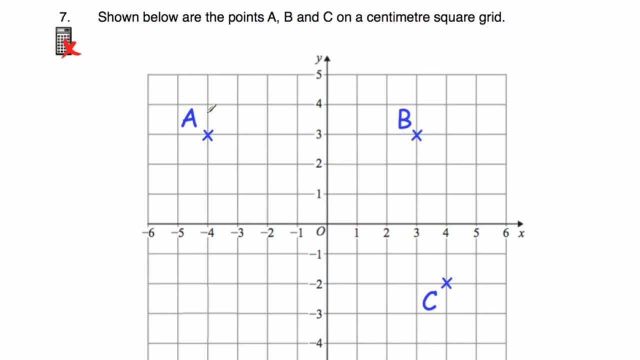 seven. okay, question number seven. so question number seven says, shown below the points a, b, c, on a centimeter square grid. so we've got this grid. it's a set of axes and each one of the squares measures one centimeter by one centimeter. and we've got a, b and c and we're told the point d. 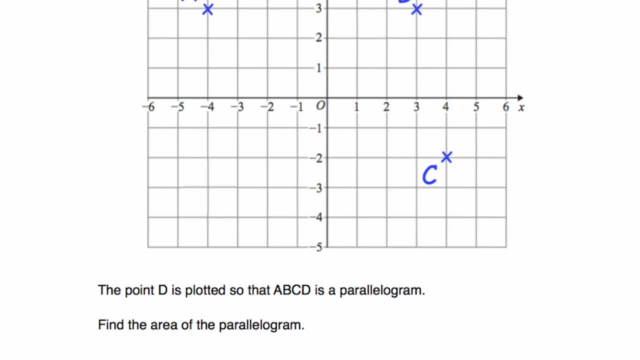 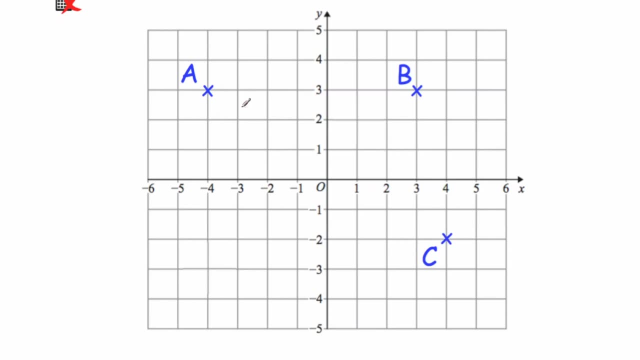 is plotted so that a, b, c, d is a parallelogram and define the area of the parallelogram. so we've got a b, c. now we need to find where d is. so remember for parallelogram that the opposite sides are parallel but they're also the same length. so if we look at the top, the length of the top is one. 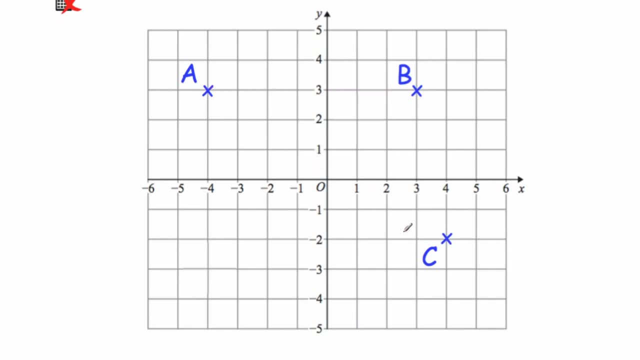 two, three, four, five, six, seven. so that means the base will have a length of seven as well. so if we go this way, seven, we go one, two, three, four, five, six, seven. that means the point d will be here. so this would be our parallelogram. it would look something like this: so we've got a. 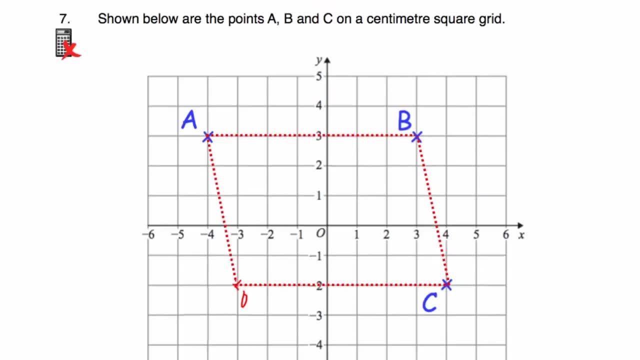 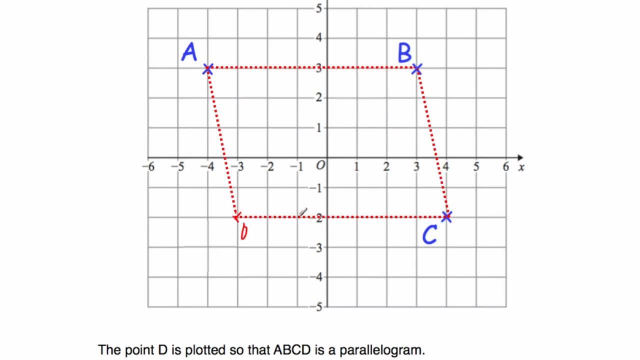 parallelogram and we've been asked to find this area, so let's find the length of the base. so in the question we're told that it is a centimeter square grid, so that means that each one of the squares measures one centimeter. by one centimeter there's going to be one, two, three, four, five, six. 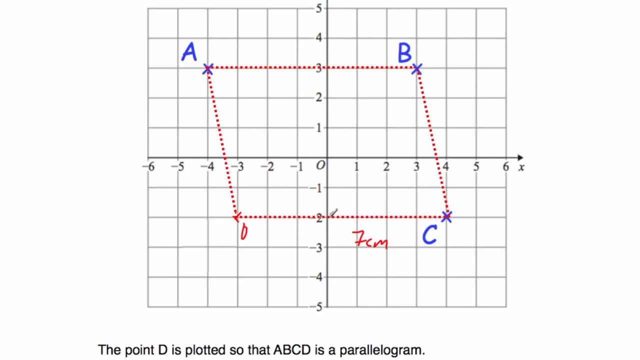 seven centimeters across and in terms of the height of the parallelogram from the base to the top, that's going to be one, two, three, four, five, so it's going to be five centimeters. so if we do seven multiplied by five, that will give us the area of this parallelogram. so the base area is equal to the base, which is: 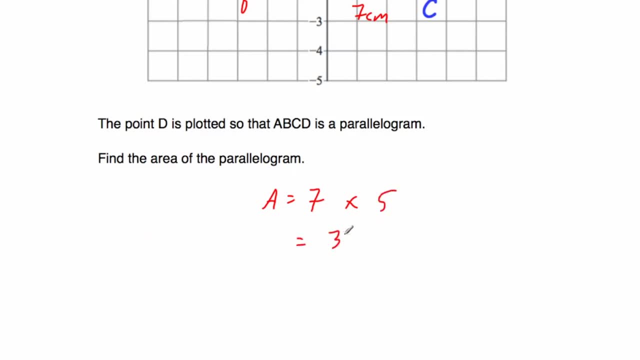 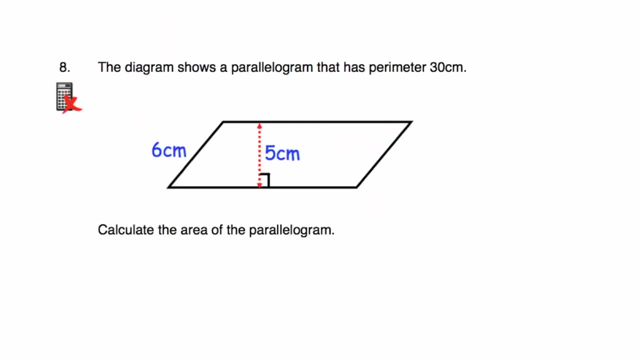 seven multiplied by the height, which is five, and seven times five, is 35 centimeters squared. and that's it. so there, the parallelogram is 35 centimeters squared. okay, our next question, question number eight. and question number eight says: the diagram shows a parallelogram with a 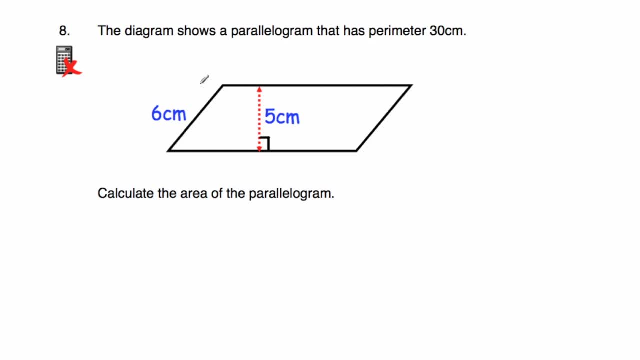 perimeter of 30 centimeters. so the perimeter of this parallelogram is 30 centimeters. so the distance around the outside is 30 centimeters. now, if the left hand side has got a length of six centimeters, that means that the right hand side would have a length of six centimeters. 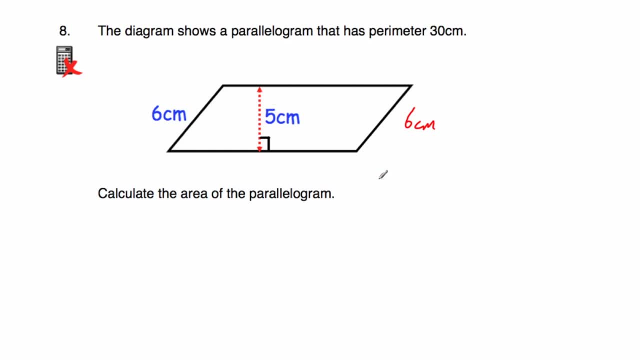 now, that's actually enough information. i would have found what the length of the top and the base would be, because we know that the distance around the outside must be 30 centimeters. so if we add six and six together, six plus six, that's equal to 12. so that means that the other two 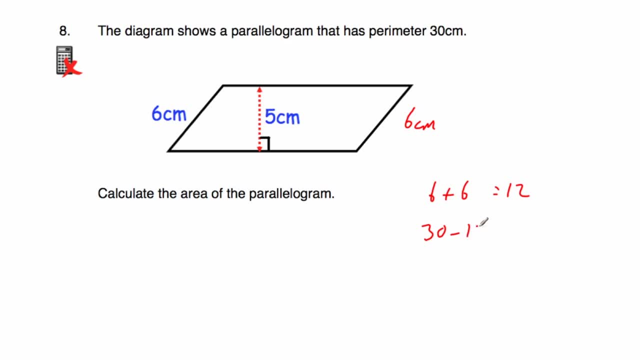 sides, whenever we add them together, must be 18, because 30 take away 12 is the length of the top, is equal to 18. so that means that when we add the two oversides together we get 18. they're the same length as each other. so if we do 18 divided by 2, that's equal to 9. so that means that the top. 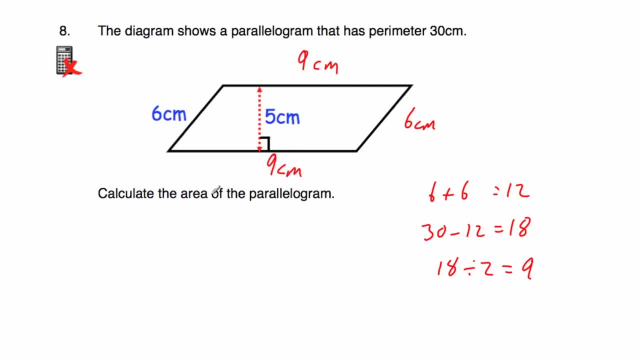 must be 9 centimeters and the base must be 9 centimeters. so we've now got our parallelogram and we've been asked to calculate its area. well, we know the base and we know the height, so the area is equal to the base times the height. the base is equal to 9, the height is equal to 5. the 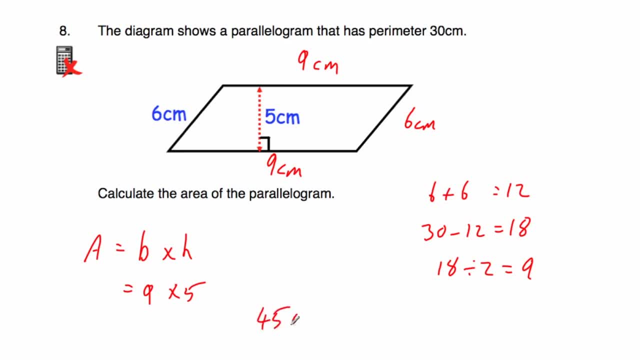 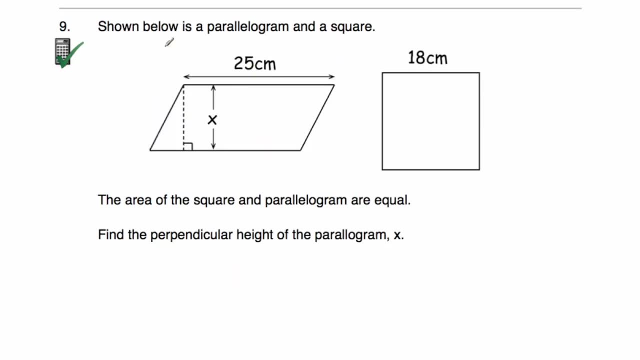 height of it. so we're going to do 9 times 5 is equal to 45 centimeters squared and that's it. so the area of this parallelogram would be 45 centimetres squared. question number nine. question number nine says: shown below is a parallelogram and a square. so we've got this parallelogram and 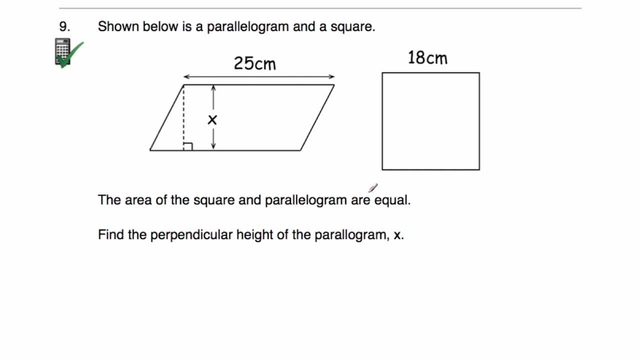 we've got this square and we're told the area of the square and the area of the parallelogram are equal and to find the perpendicular height of the parallelogram. so let's find the area of the square to begin with, because we know the square is 18 centimeters wide. 18 centimeters. 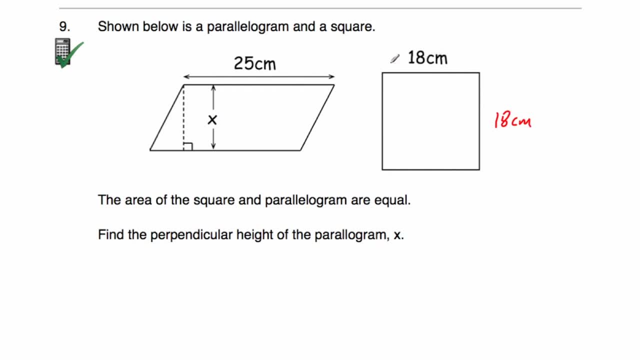 tall and so on. it's 18 by 18, so we want to find this area. we're going to multiply the length by the width, so we're going to do 18 times 18, so we're going to do 18 multiplied by- and it's a calculator question, so that's quite nice, and the answer would be equal to 324 centimetres. 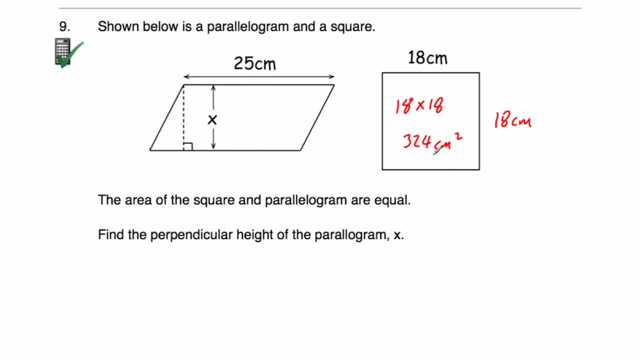 squared. So the area of this square is 324 centimetres squared. but we're told in the question the area of the square and parallelogram are equal. so that means the area of this parallelogram will also be 324 centimetres squared. So now we know the area of the parallelogram. we 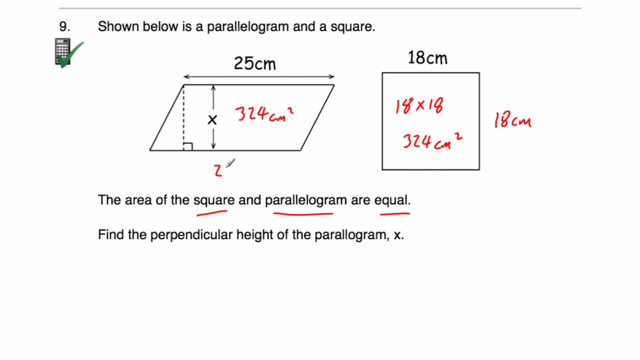 can work out the height of the parallelogram, because we know that the base, which is 25 centimetres, the same as the height. 25 multiplied by the height would give us 324.. So if we do 324 divided by the length of the base, 25, we can find the height of the parallelogram. So 324 divided. 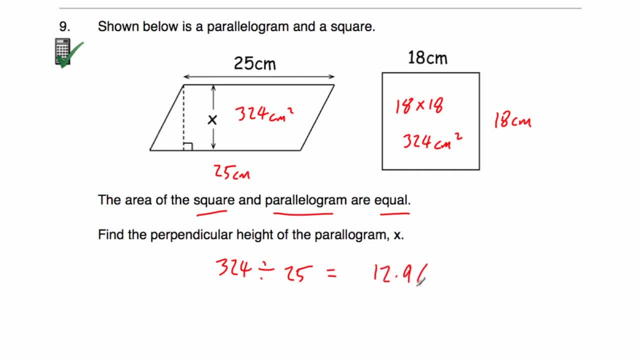 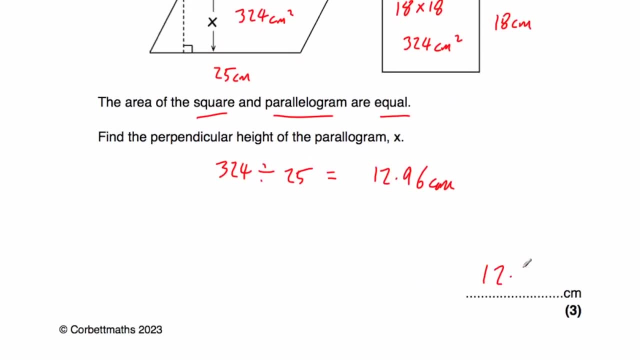 by 25 is equal to 12.96 centimetres, and that's it. So the height of this parallelogram would be 12.96 centimetres. Okay, question number 10.. So question number 10 says Dylan creates a logo. 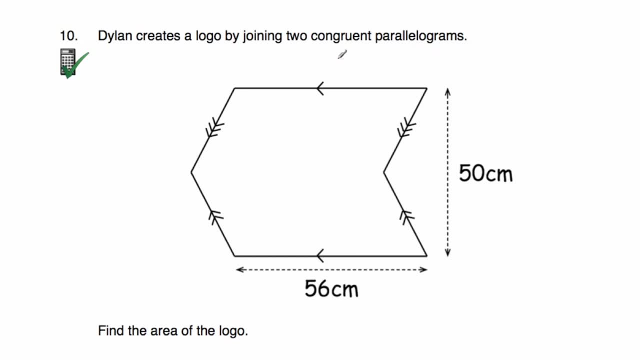 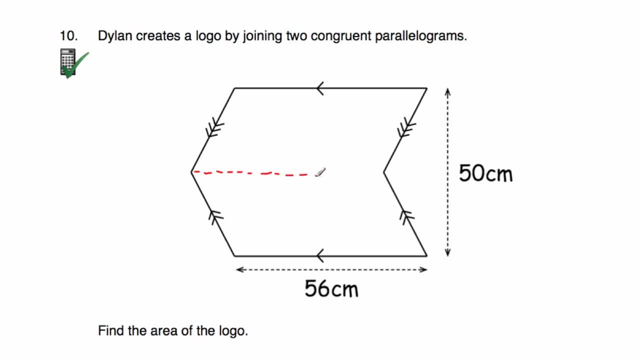 together, We actually divide them. You can see here, if we divide the shape into two, you can see there's a parallelogram on the top and a parallelogram below. We've been asked to find the area of the logo. So if we find the area of one parallelogram, we can then double it to get the 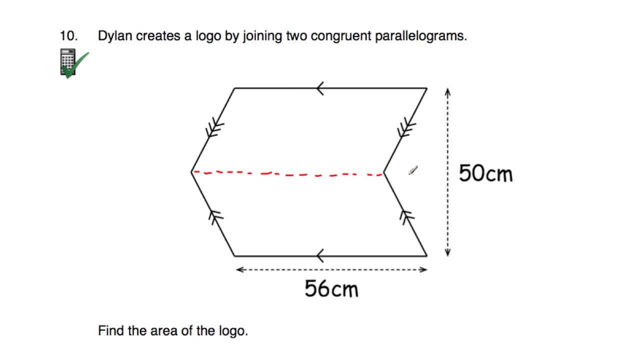 area of the whole logo. So let's consider the area of one of the parallelograms. So let's consider one of them. Let's consider this parallelogram on the bottom here, This parallelogram here, it's got a length for a base of 56 centimetres. Now, if we know the height of this, 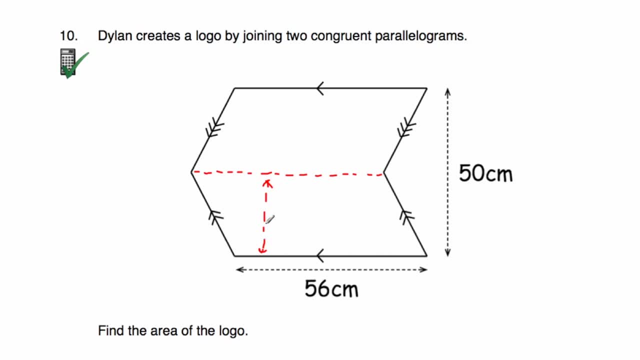 parallelogram. we can find this area by doing 56 multiplied by the height. Now, the height of the parallelogram. well, the height of both of them is 50 centimetres. So if we do 50 divided by 2, that's. 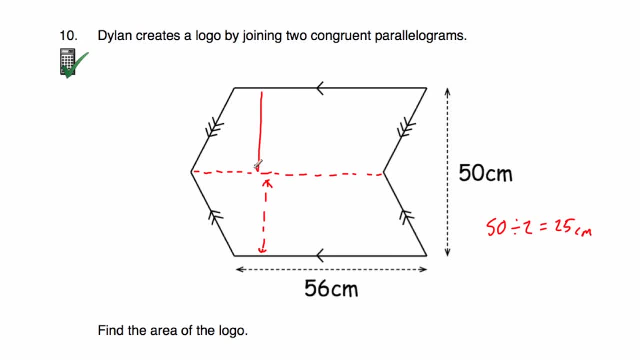 equal to 25 centimetres. So that means that this parallelogram here has got a height of 25 centimetres, and it also means that this parallelogram here has got a height of 25 centimetres. So now we know the base of the parallelogram and the height of the parallelogram if we times them. 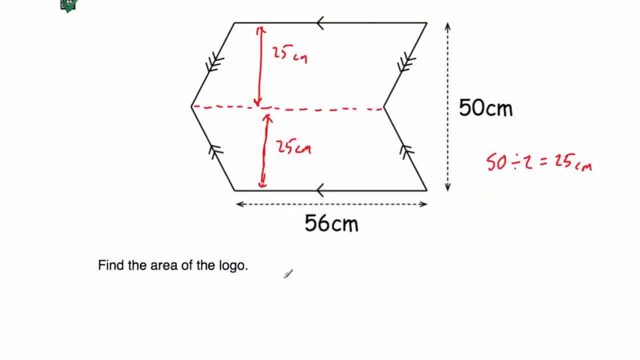 together we can find the area of the parallelogram. so let's do: area equals base, which is 56, multiplied by the height, which is 25. it's a calculator question, so that's quite nice. so 56 multiplied by 25 is equal to 1400 centimeters squared. now that was the area of just one of the parallelograms. 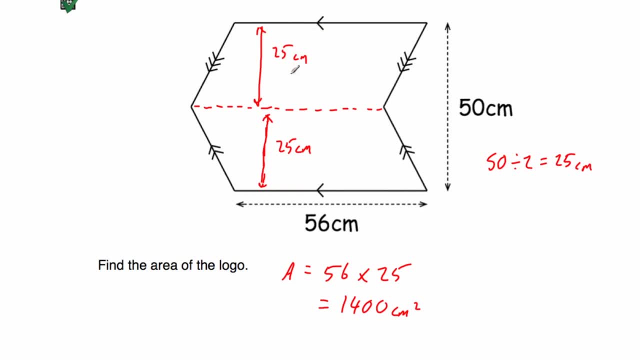 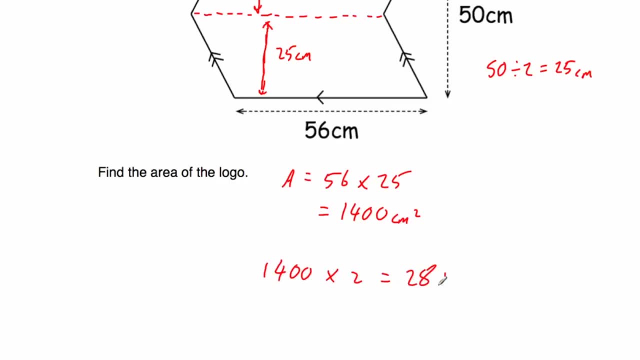 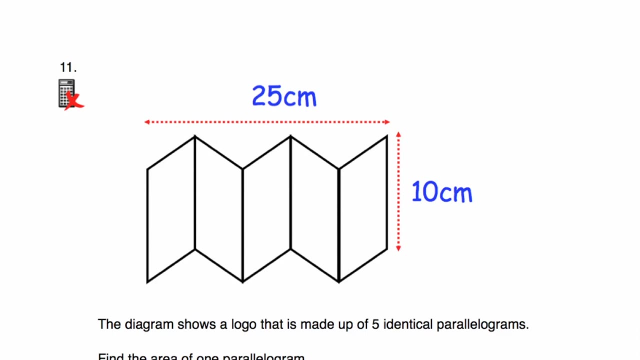 this area of this one at the bottom. now we want to find the area of the whole logo, but there's two parallelograms, so we just need to double this area. so 1400 multiplied by 2 is equal to 2800, so the area of the logo is 2800 centimeters squared, and that's it, okay. our next question. 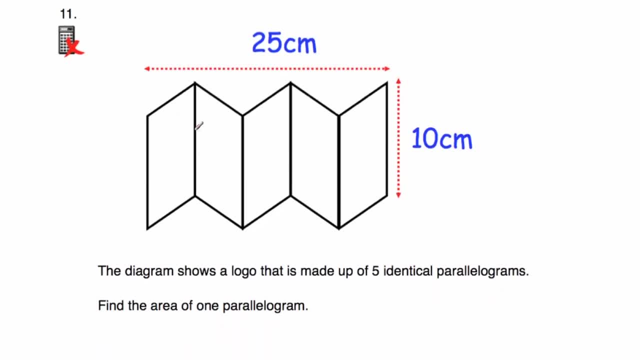 question number 11. so question number 11 says the diagram shows a logo that is made up of five identical parallelograms. so we've got one, two, three, four, five parallelograms and we've been asked to find the area of one of the parallelograms. so to find the area of one of the parallelograms, 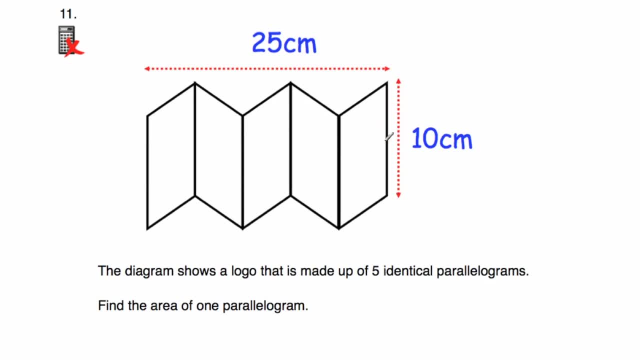 such as this one. here, what we need to do is we need to do the base multiplied by the height. now, if we turn our head sidewards here, we can see the base is going to be 10 centimeters and the height is going to be 10 centimeters. so we need to do the base multiplied by the height. 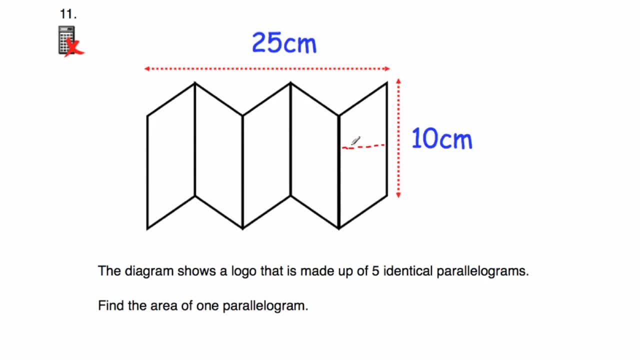 would be this distance here. so we can just find the height of this parallelogram, this distance. we can then do 10, multiply with that to find the area of one of these parallelograms. now the whole length of the whole shape is 25 centimeters and the parallelograms are identical. that means the 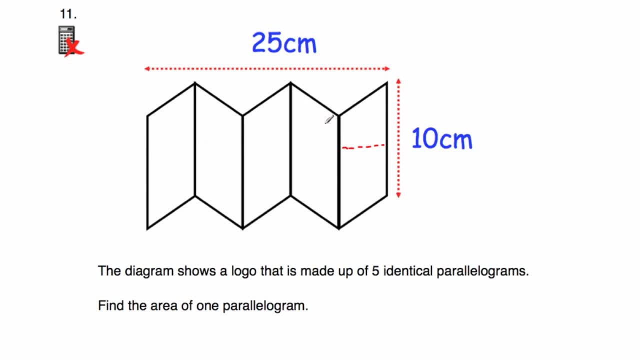 height or the width of each of them. the width of each of these parallelograms would have to be the same. so if we do 25 divided by 5, that would be equal to 5 centimeters. so that means that each of these parallelograms has got a width of 5 centimeters. so that's going to be 5 centimeters. 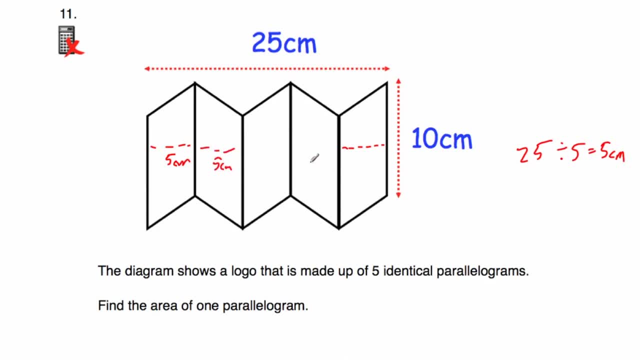 across, that's going to be 5 centimeters across and so on, and it means that our parallelogram we were looking at here has got a width of 5 centimeters also, and if we turn our head sidewards, the base would be 10, the height would be 5, and then we just times them together to get 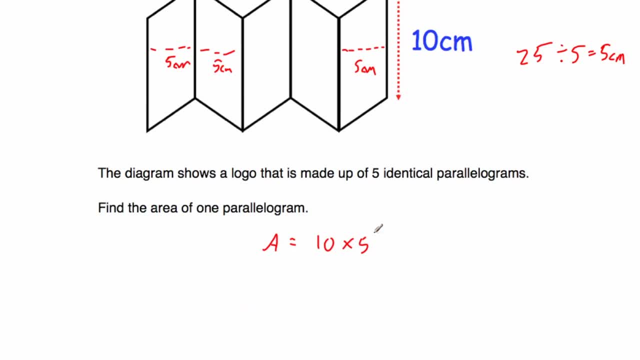 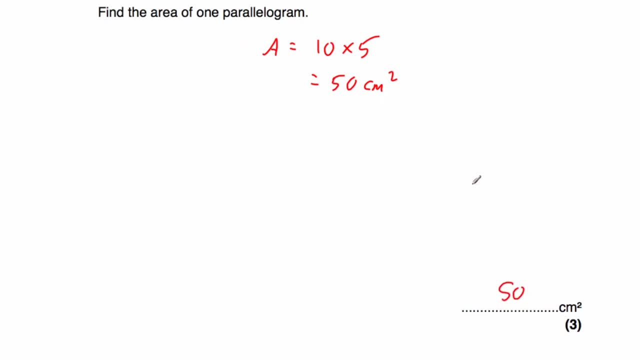 the area. the area is equal to the base 10 times the height, 5, and that's equal to 50 centimeters squared. so the area of one of the parallelograms is 50 centimeters squared and that's it okay. question number 12. question number 12 says a shape is made from four congruent. 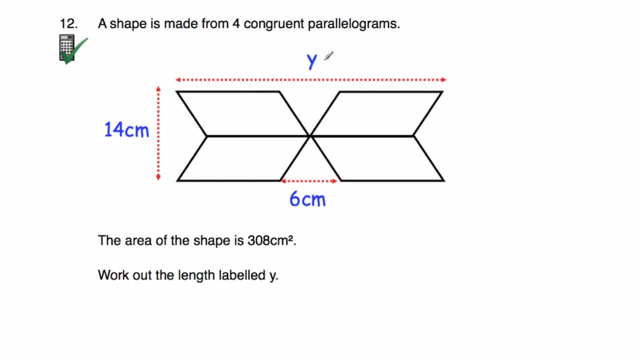 parallelograms. so congruent means identical, so it means they've got the same shape and size and area. and we've got this diagram and we're told that the height of this shape is 14 centimeters. we're told that the whole length of it is y and at this distance is 6. so if we have a look at it, 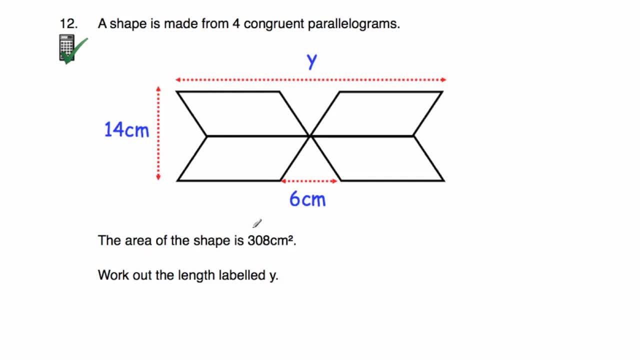 we've been asked to find this distance here, but we've been told that the area of the shape is 308 centimeters squared. so the shape consists of four identical parallelograms. so if we divide the total area by four, we can find the area of each one of these parallelograms. so if we divide the total, 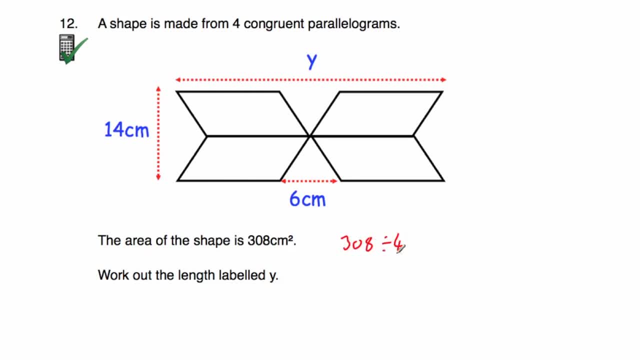 these parallelograms. So we're going to do 308 divided by 4, and when we do 308 divided by 4 we get that's equal to 77 centimetres squared. So the area of each one of these parallelograms- 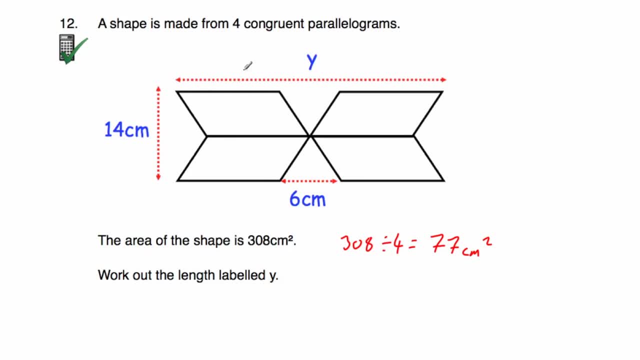 is 77 centimetres squared. Now we want to find this length, y. Now if we know that this distance is 6, that means the distance to the top here is also equal to 6 centimetres. So if we can find out what the length of one of the parallelograms is, we can do the length of one of them plus 6. 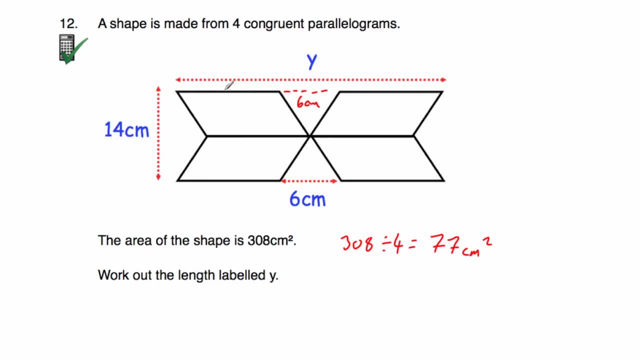 plus the length of another one. So we really need to find this length, this length of this parallelogram, the length of the base or the length of the height, and that will then mean that we can find the total distance y. Now we know the area of each one of them is 77 centimetres squared. 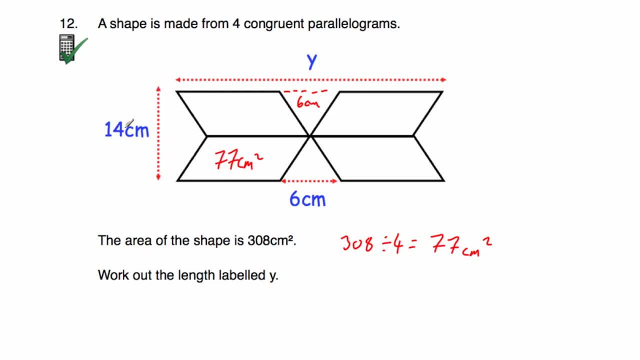 Now let's consider the height of them. The height of the whole shape is 14 centimetres, so that means the height of each one of them is half of that, which is 7 centimetres. So the height of each one of them is 7 centimetres. So remember to get the area of a parallelogram. we do the base times. 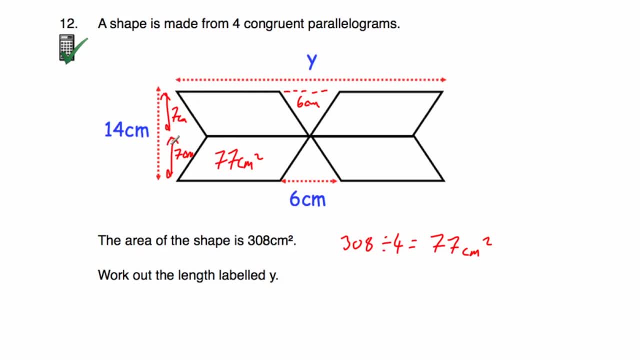 the height And that gives us the area. So that means that this 7 multiplied by how long it is gives us 77. So if we do 77 divided by 7, the height of it, that will give us the length of each one of the. 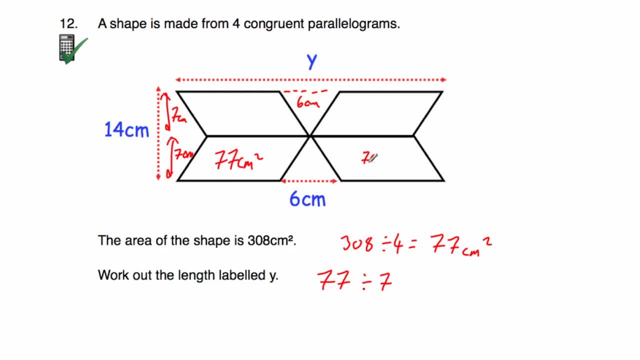 parallelograms, because if we have a look at one of them, we know its area is 77 centimetres squared. We know that its height, the top to bottom, is equal to 7 centimetres and that means that 7 times. 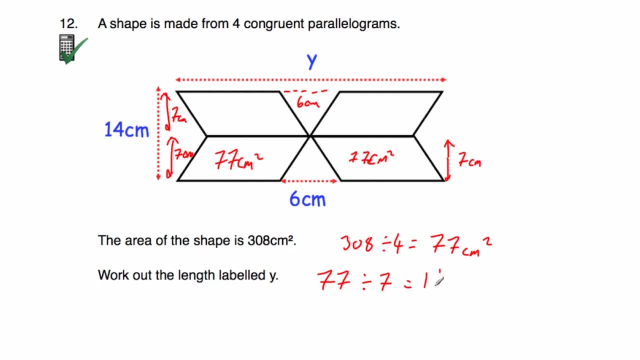 something will give us 77.. So 77 divided by 7 is equal to 11.. So it means that each parallelogram is 11 long or wide, or the base of it is 11, and the height of each one of them is 7 centimetres. 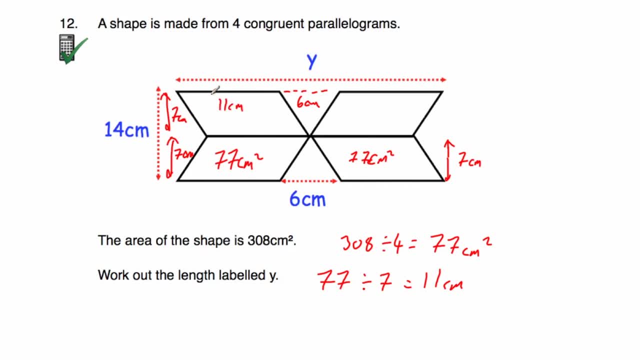 Now we want to find this length y, So that's going to be 11 centimetres, that distance plus 6 plus 11.. And if we do 11 plus 6 plus 11, we will get the length of the whole shape. So 11 plus 6 plus 11.. 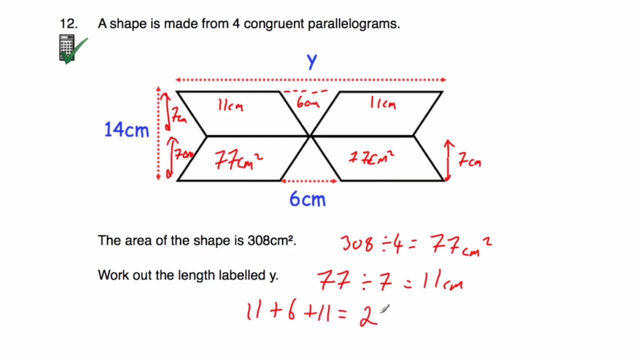 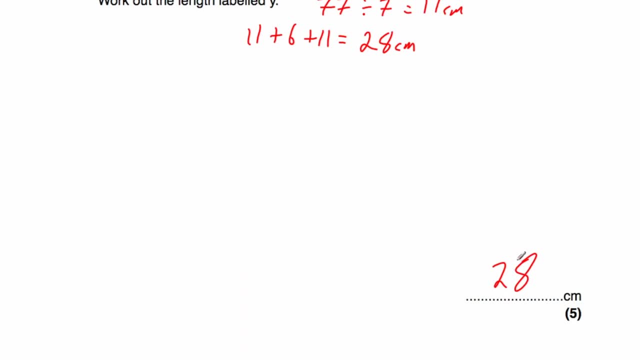 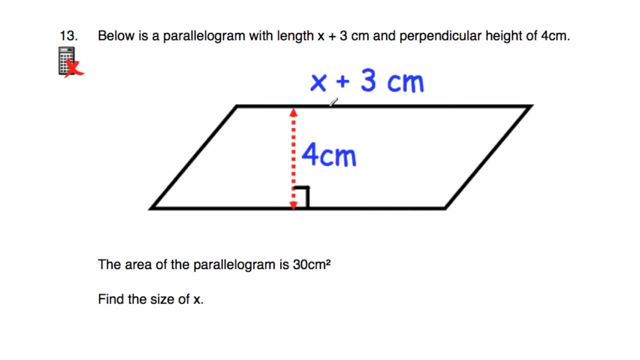 11 plus 6 is 17 plus 11 will be 28.. So that means that this whole shape has got a length of 28 centimetres, And that's it. Okay. let's have a look at questions, Question number 13.. So question number 13 says: below is a parallelogram with a length of x plus 3 centimetres. 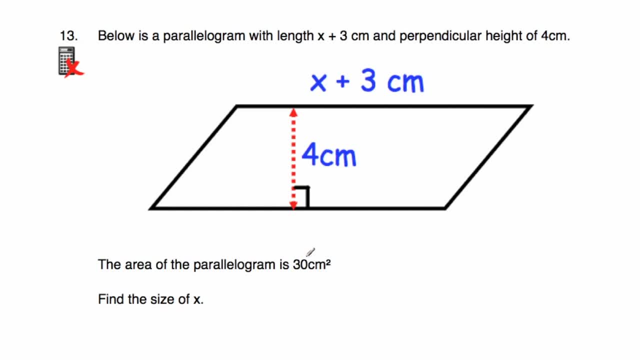 and a perpendicular height of 4 centimetres And we're told the area of the parallelogram is 30 centimetres squared and we've been asked to find x. Now there's two different ways you can do this question, or two different ways. 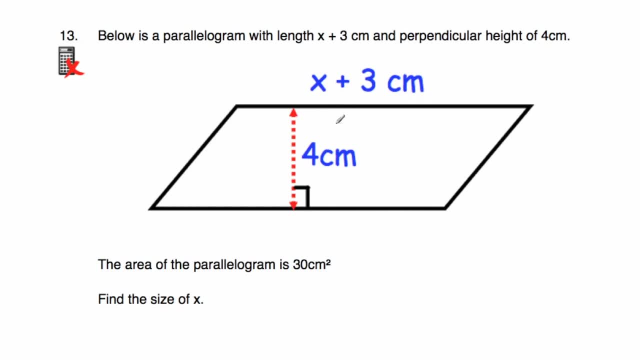 I can pick off to do this question and I'm going to do both approaches now. So the first approach is to work using the algebra To find the area of the parallelogram. we do the base times the height, So the base is the. 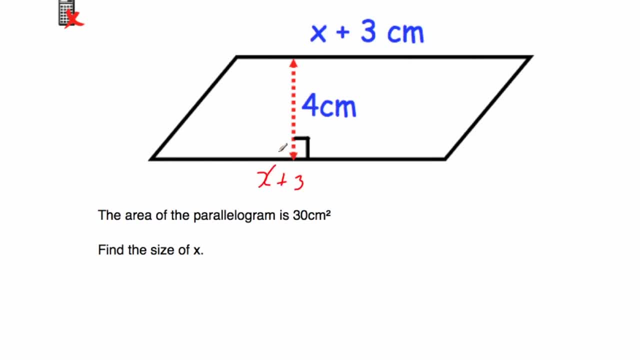 same as the length here. So that's going to be: the base is x plus 3 and the height is 4.. So if we times this together, we will get the area, So 4 multiplied by x plus 3.. Now, whenever we are multiplying x plus 3 by 4, we just put the x plus 3 in a bracket and we put a 4 in front. 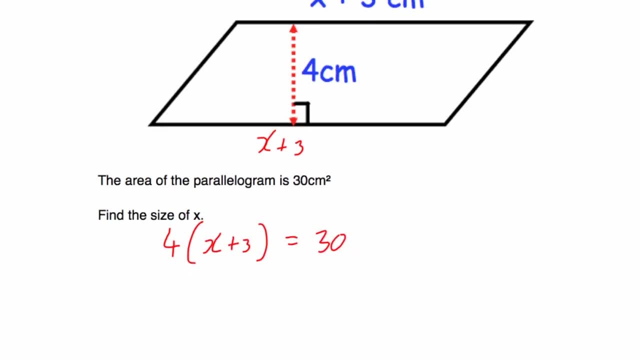 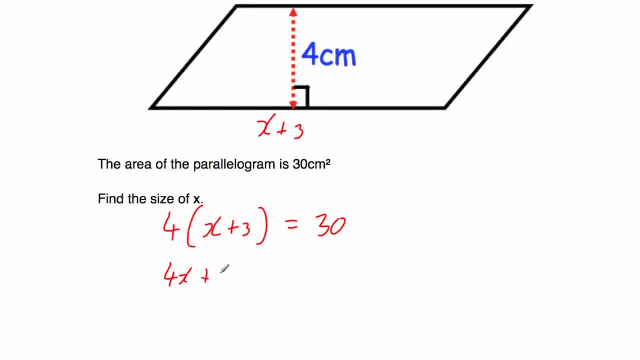 And that will be equal to 30 centimetres squared, or 30. And if we solve this equation, we can find x, So expand on our bracket. So 4 times x is 4x and 4 times 3 is 12.. So 4x plus 12 is equal to 30.. 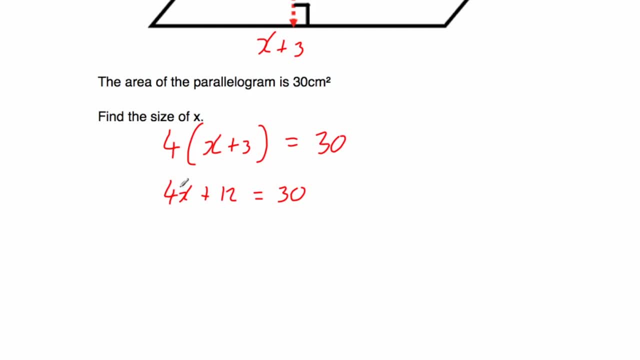 Now we just want to solve this equation, So we want to get the x on its own. So we don't want this multiplied by 4 and we don't want this plus 12.. So let's get rid of the plus 12 by taking away 12 and taking away 12.. So 4x plus 12, take away 12.. We just leave this for 4x, And on the right hand side we have 30. Take away 12 is equal to 18.. 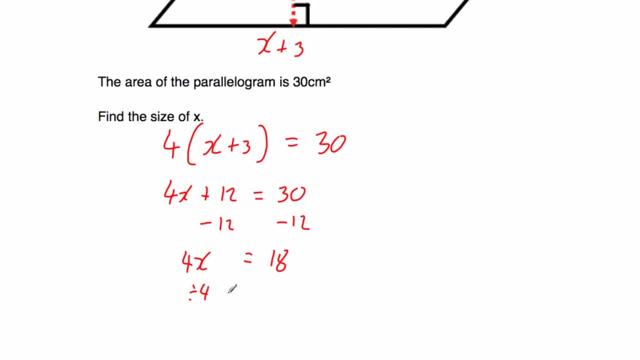 Now we've got 4 times x. We don't want this multiplied by 4.. So let's divide by 4 and divide by 4.. 4x divided by 4 is equal to x, And 18 divided by 4.. Well, that's equal to half of 18 is 9.. Half of it again is 4.5.